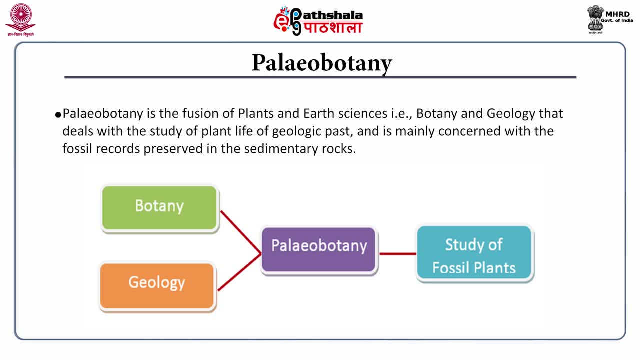 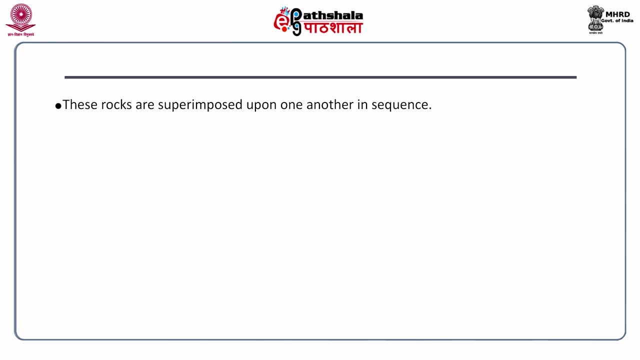 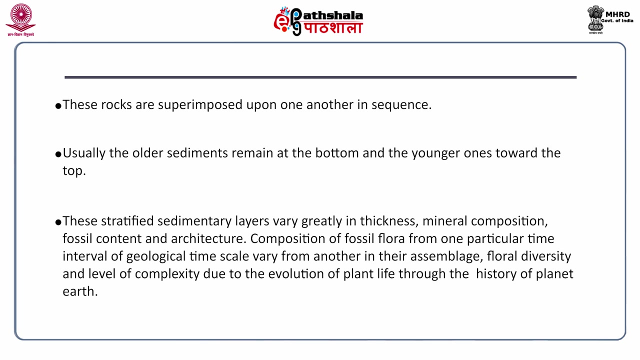 that are preserved in the sedimentary rocks. These sedimentary rocks are superimposed on one another in sequence. Usually the older sediments remain at the bottom and the younger ones toward the top. These stratified sedimentary layers vary greatly in thickness. mineral 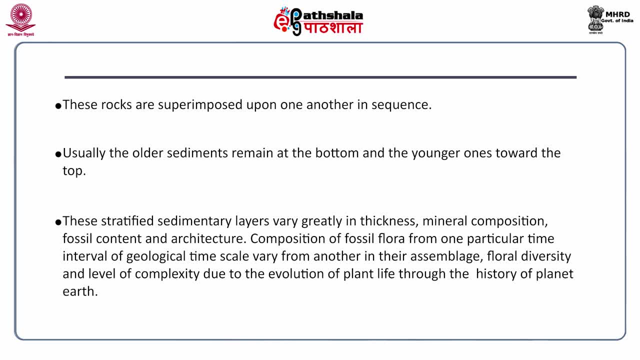 composition, fossil content and architecture, So these may be different based upon these things. So this is the study of flora from one particular time. interval of geological time. scale vary from another in their assemblies, floral diversity and level of complexity, and that is due to. 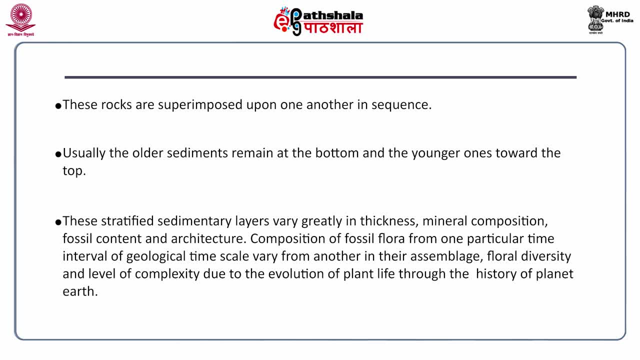 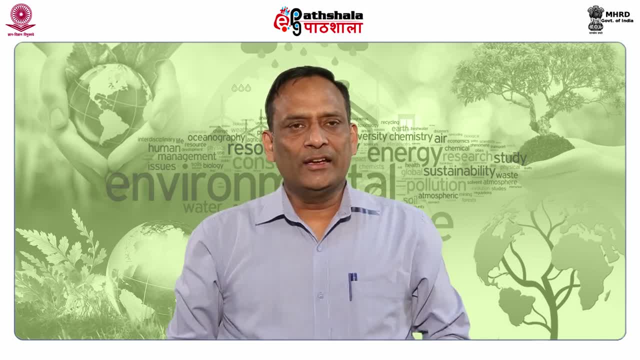 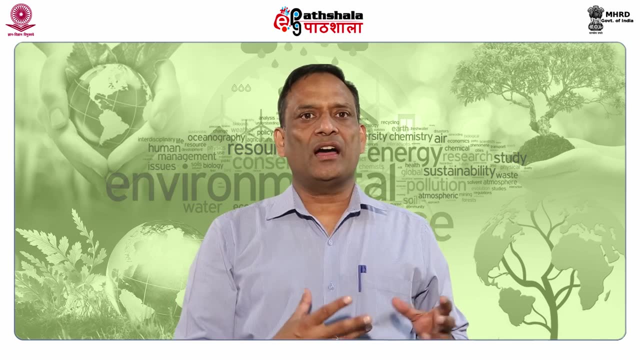 evolution of plant life through history of planet earth. So basically, this is the study of fossil plants. So we must know what are the fossils? Fossils are the relics of the past and are the evidences of prehistoric life of plants. 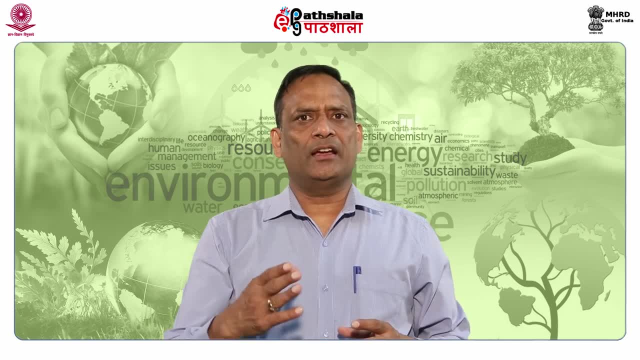 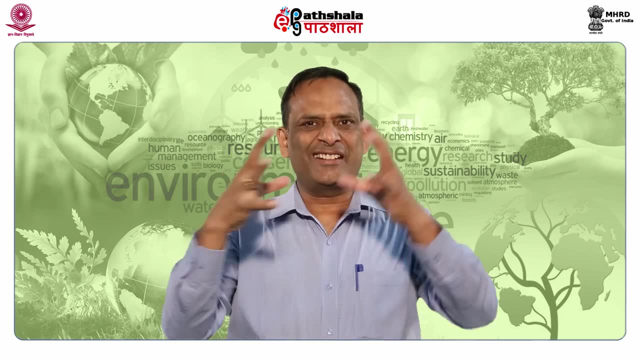 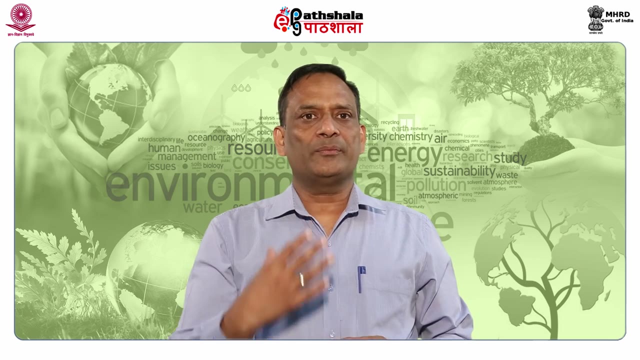 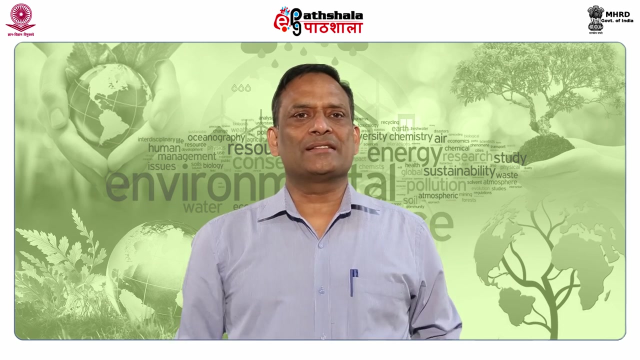 We will be studying about fossils in paleontology in detail, but the fossils of the plants are studied in paleo botany and similarly, when we study the fossils of the animals, they are studied under paleontology has appeared here- paleontology. paleontology is nothing but the study of fossils of animals. 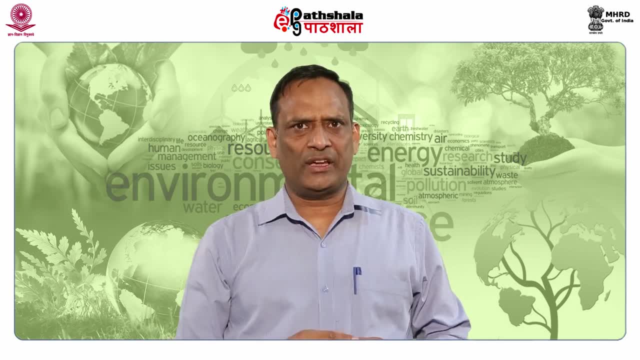 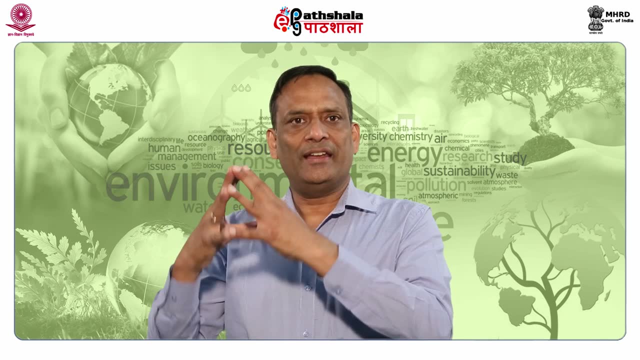 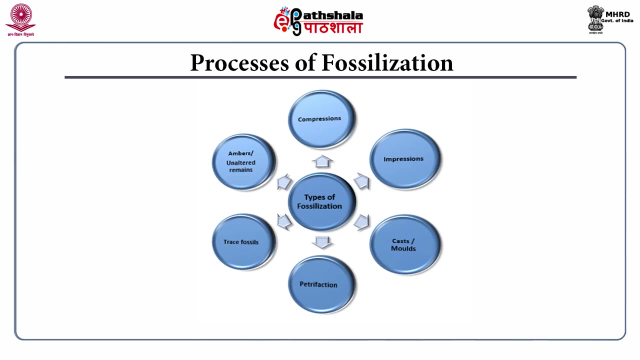 And these fossils of plants, as well as that of animals, are considered as direct or indirect evidence of past life. There are number of processes which are responsible for the formation of fossils, and these processes are shown here in this graph. These processes of fossilization include compression, impression, cast and molds, petrification, trace fossils and unaltered 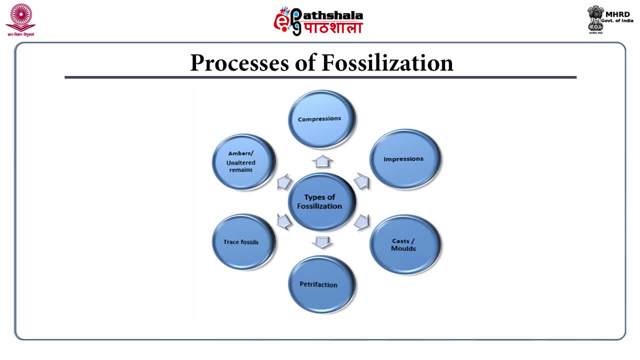 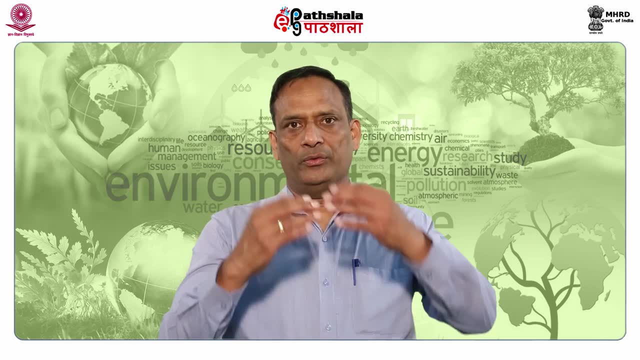 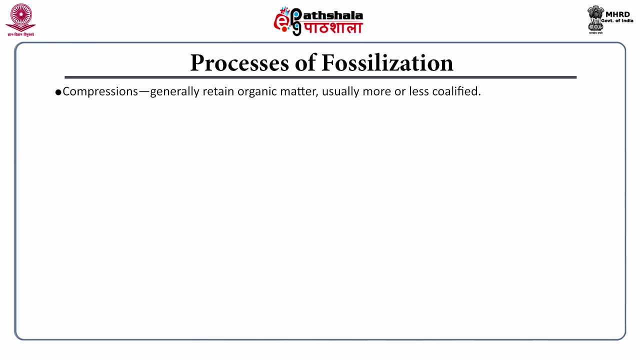 remains. So these are the different processes by which fossilization take place. Now we will try to learn little bit about these processes. Now we will talk about each process of fossilization. First one is compression. Compression generally retain organic matter, usually more or less qualified Means, we can say the coals which 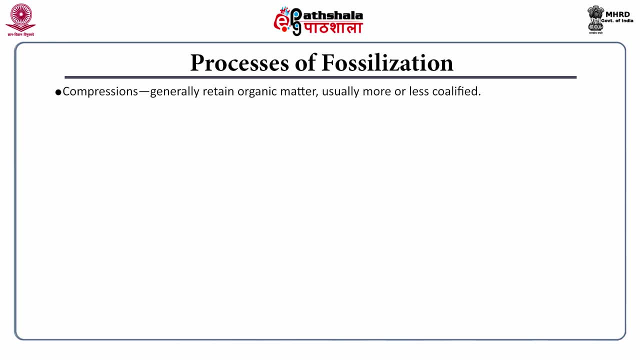 we have. they are the result of compression process, of fossilization, Then impressions, as the name are indicating. Here we only have the imprints of plant remains. Basically these imprints of plant remains are preserved in the sedimentary rocks. Impression fossils are divided of any organic matter. 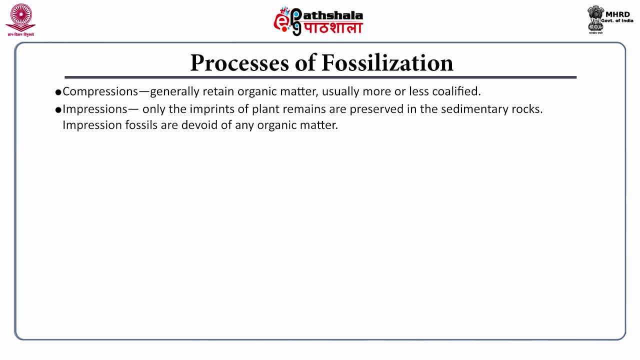 In case of compression we get organic matter, whereas in case of impression we don't have any organic matter, we just have imprints. Then cast and molds In cast and molds, basically a cast. result: that how a cast is formed when sediment is deposited into cavities left by. 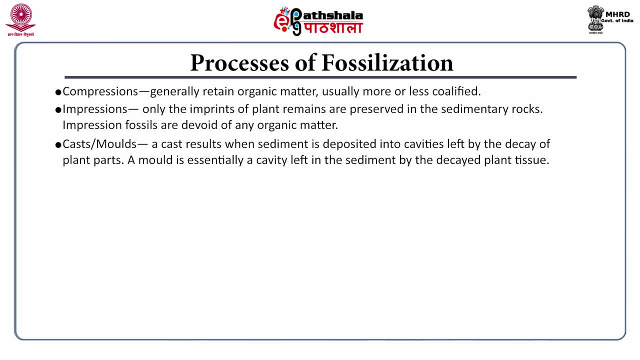 the decay of plant parts. A mold is essentially a cavity left in the sediment by the decayed plant tissue. Then petrification or permineralization. permineralization occurs when the plant tissues are in filtered with minerals in cell lumens and intercellular spaces, Thus preserving internal structures. 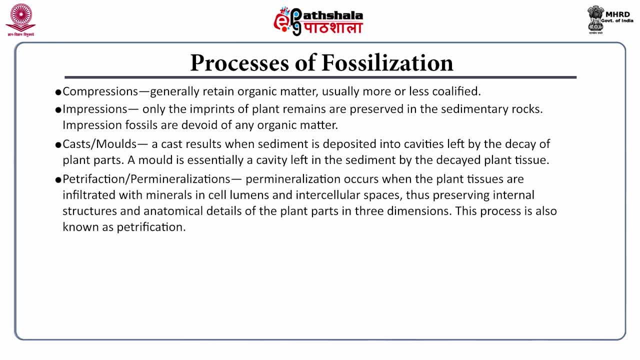 and anatomical details of the plant parts in three dimension. This process is also known as petrification. Then trace fossils. Trace fossils are any indirect evidence of past life, records, behavior and ecological constraint, For example tracks, tracks, trails, burrows, coprolites, Basically. 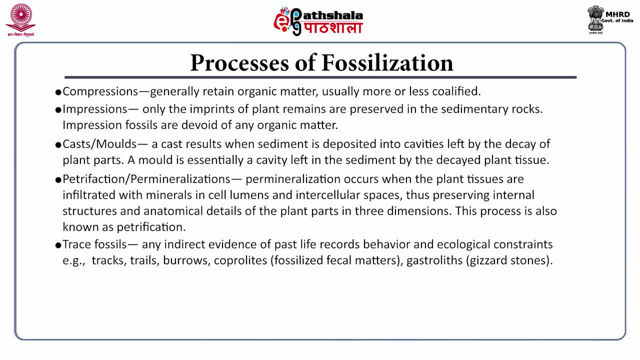 coprolites are nothing but fossilized features. Then canola- Canola is a typical matter- Then gastroliths- Gastroliths are geyser stones- Then unaltered remains and embers, Basically unaltered remains. these are entombed in the 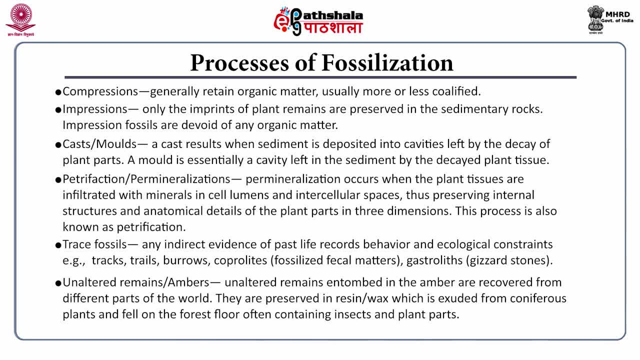 ember or recovered from different parts of the world. They are preserved in resin and wax which is exuded from coniferous plants and fell on the revealed from the top of the mountain or forest. The remaining embers are then 퓄, Abrahamic. 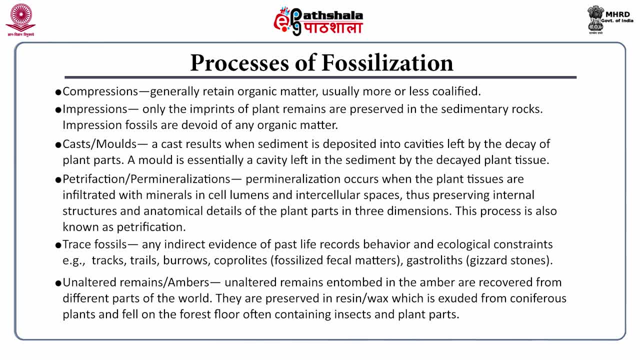 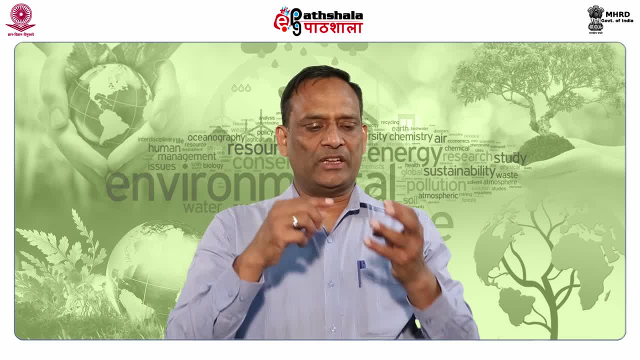 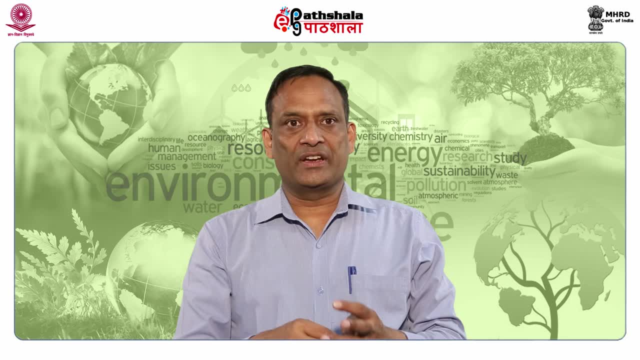 forest floor, often containing insect and plant parts. So these were the different processes. I am again repeating these processes. One of them is compression. In case of compression, we get organic matter, then impression, then permineralization, then unaltered fossils, etc. 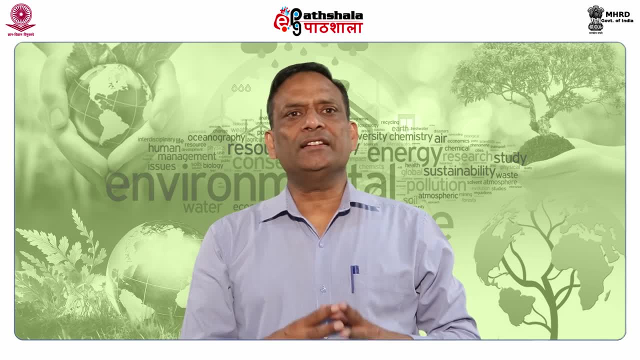 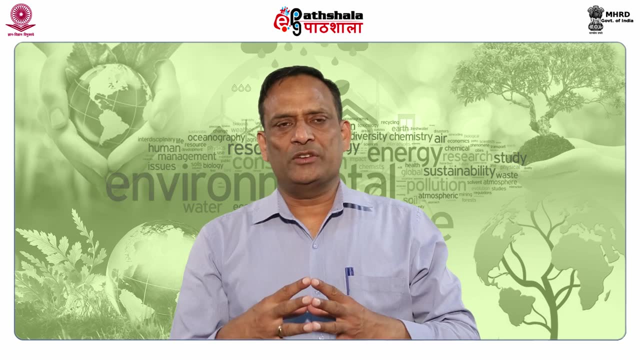 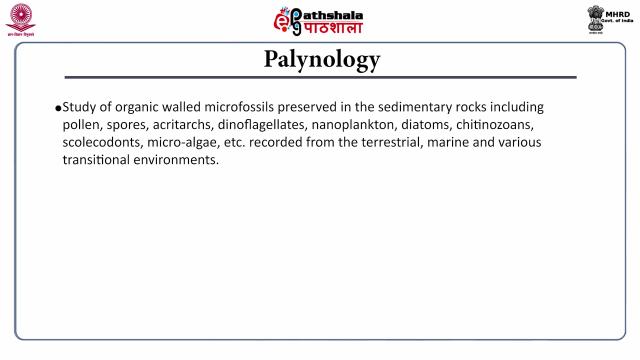 So these were different processes. Then there is a another term that is palynology, that is used in paleobotany. What is palynology? Palynology is the study of organic wild microfossils preserved in the sedimentary rocks, and these 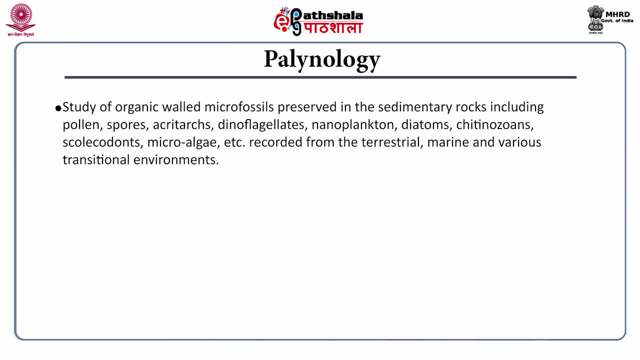 microfossils includes mainly pollen grains, spores, acrytrachs, dinoflagellates, nanoplankton, diatoms, chitinogens, then scolicodonts, microalgae, etc. So means in general, you will find in the books that the study of the pollen grains 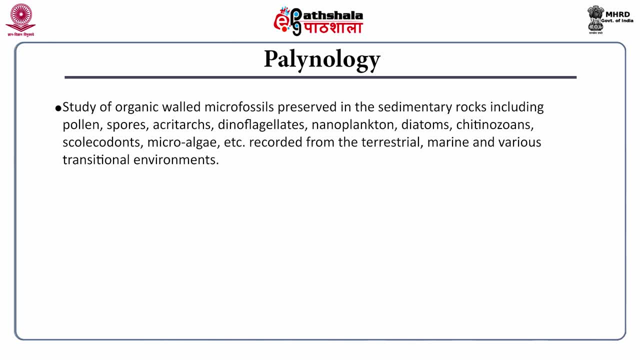 and spores is called as palynology. These all are recorded from the terrestrial, marine and various environments. So here we can say that paleobotany includes The study of the terrestrial plants, as well as marine autotropes, due to their small size. 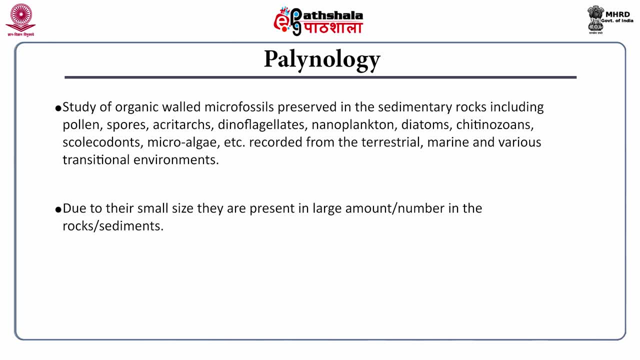 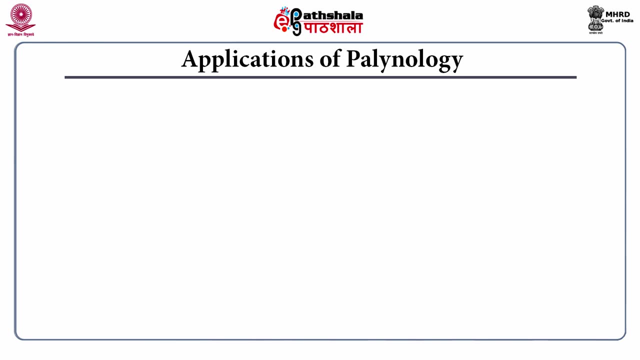 they are present in large amount and number in the rocks and sediments. They are documented almost in the entire range of geological time scale, that is, from pre-Cambrian to the Holocene. Now, what are the applications of palynology? Palynology is one of the subdivisions, as I have told earlier, paleobotany, and it can 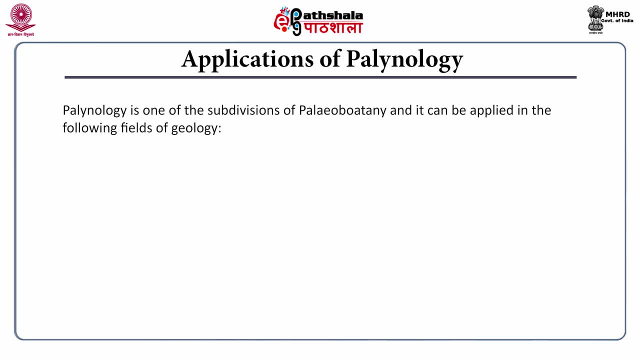 be applied in the several fields of geology. Let us see where palynology can be applied. So one field is biostratigraphy. In biostratigraphy, palynology is largely used in biostatigraphic studies for demarcation. 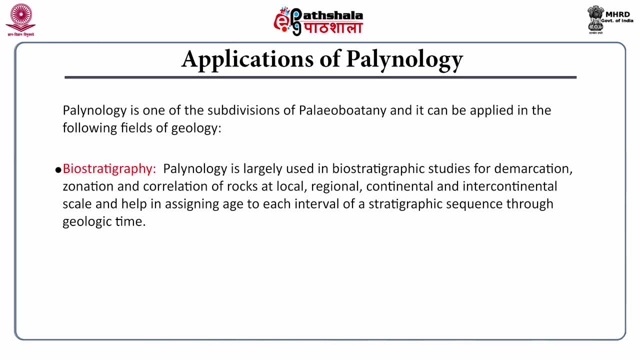 zonation and correlation of rocks at low altitude, So this is a very important field. It is used in local, regional, continental and intercontinental scale. This also helps in assigning age to each interval of a stratigraphic sequence through geologic 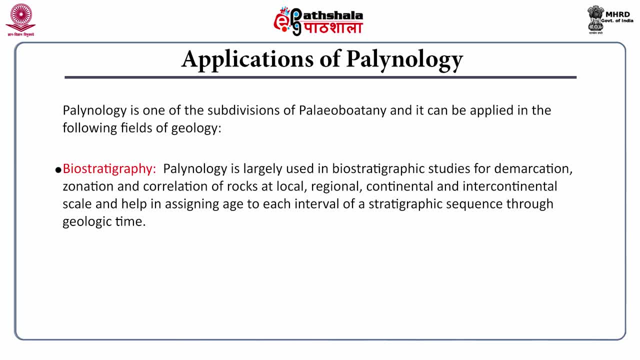 time. There is another application of palynology, and that is in the field of paleoecology. This palynology can be used to reconstruct paleo-vegetational scenario in any part of the world and to understand paleo-geographic conditions, in addition to understanding past. 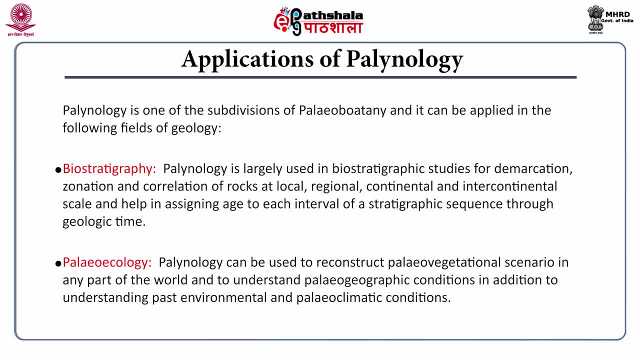 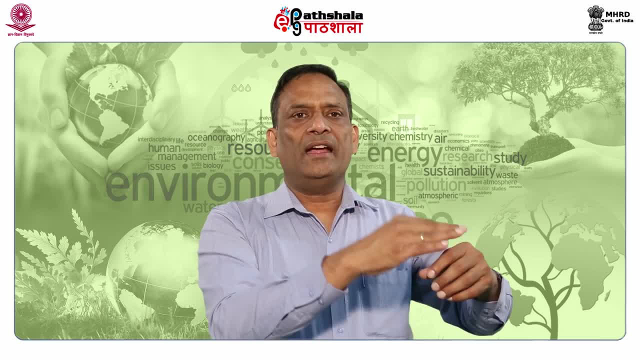 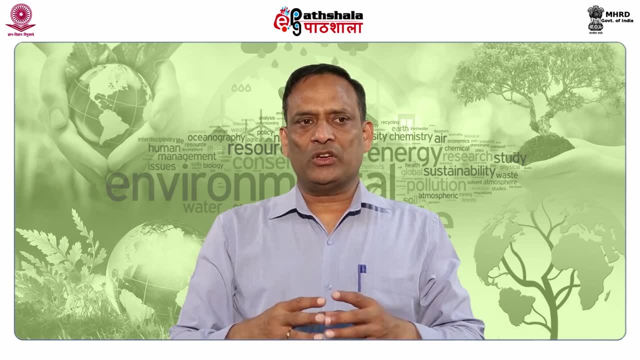 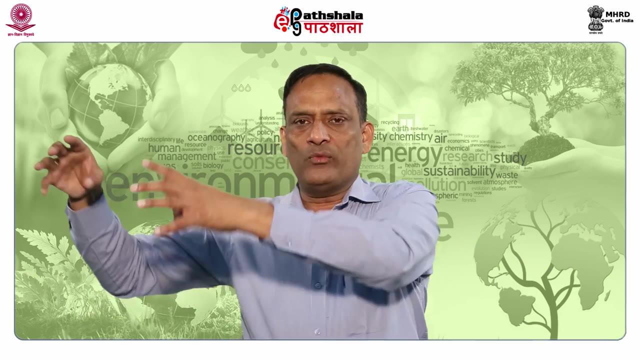 environmental and paleoclimatic conditions. For example, in one area we find the remains of the plants and that plant is existing today also. So presuming that because this plant existed in past also And existing today also, it means the environment in which this plant is growing here today. 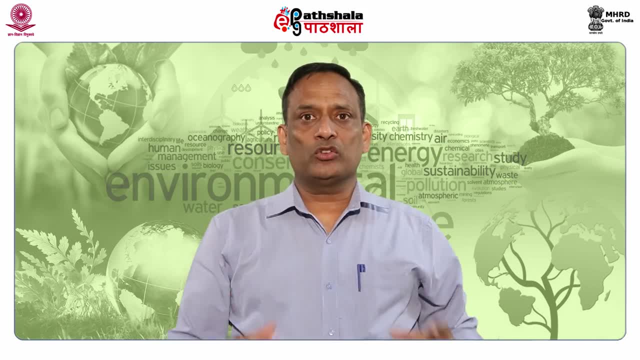 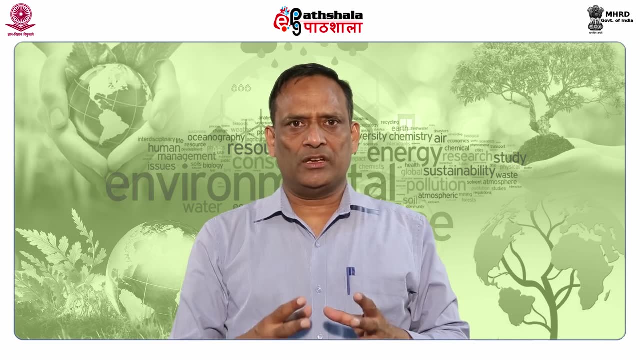 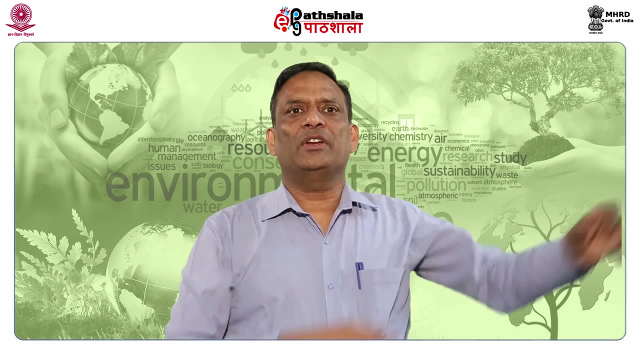 the same environment was existing millions of years ago. So means what we can find out, we can trace back that what based upon this paleo botany or based upon this plant fossil, that at that time what kind of climate was existing. 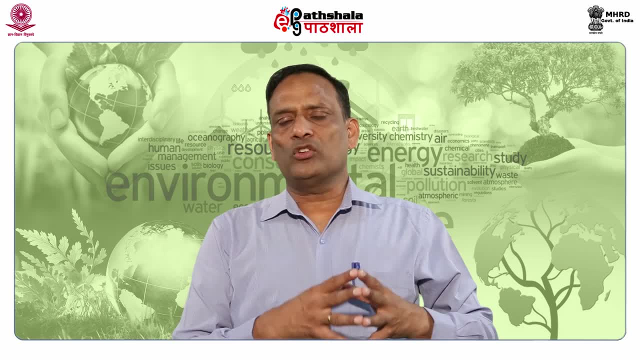 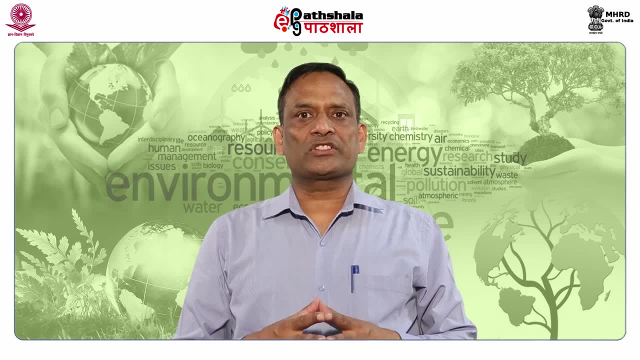 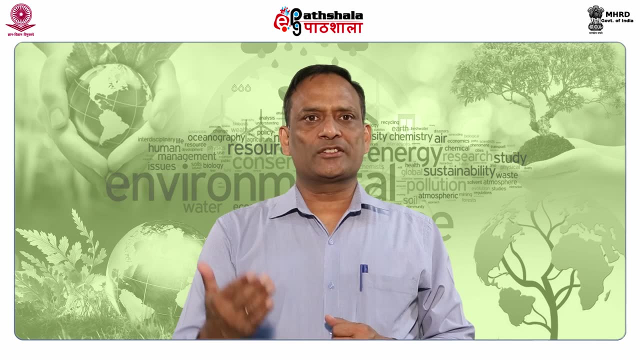 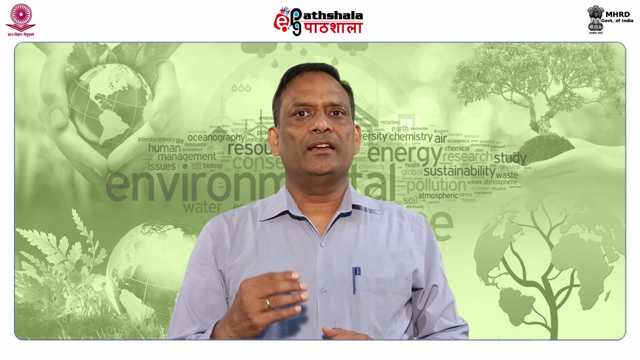 is in petroleum exploration. The main source material for hydrocarbon generation is organic debris. you know that all That includes fossil spores and pollen, phytoplankton, marine and terrestrial algae, as well as lipid rich land plant remains Direct applications of these distillation. 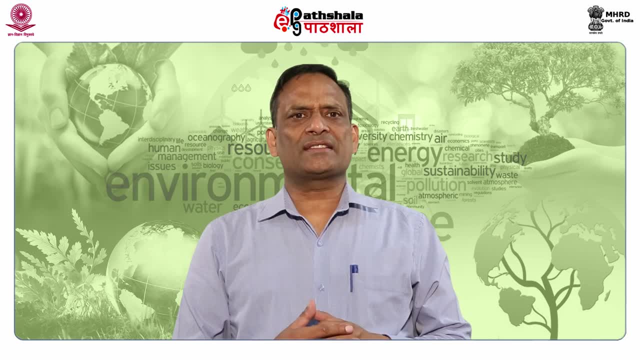 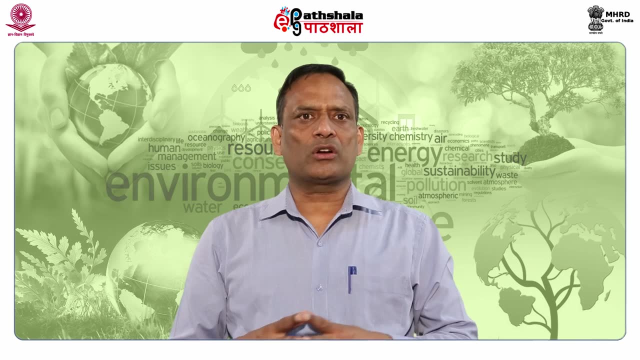 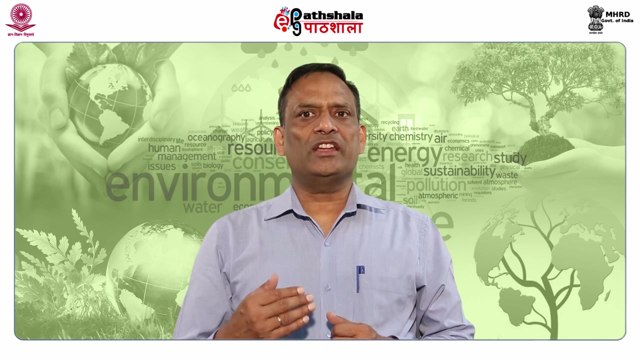 Part of this disperse organic matter. This also known as the sedimentary organic matter, lies in identifying hydrocarbon source rock evaluation and potential of the sequences while estimating their type, quantity and maturity in the sedimentary rocks. These are there are number of organic matter. maturation scales for measuring the degree. 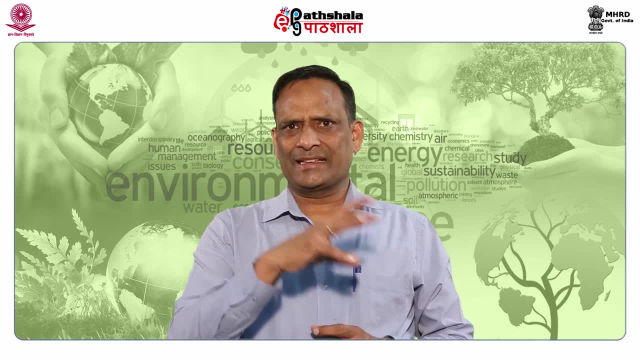 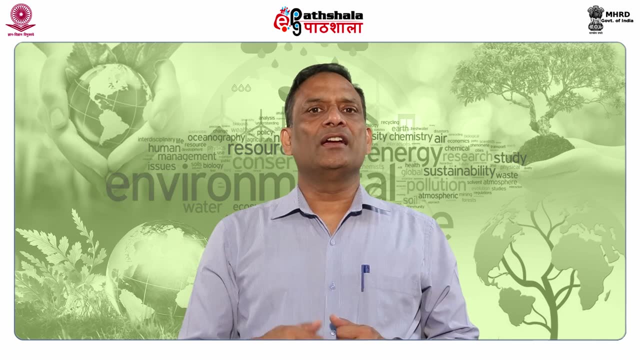 of thermal alterations. This has been also known as sedimentary organic matter. What makes a rock like this so abstract? alteration index. In short, this thermal alteration index is called as TAI values for delineating hydrocarbon source potential of sedimentary sequence. 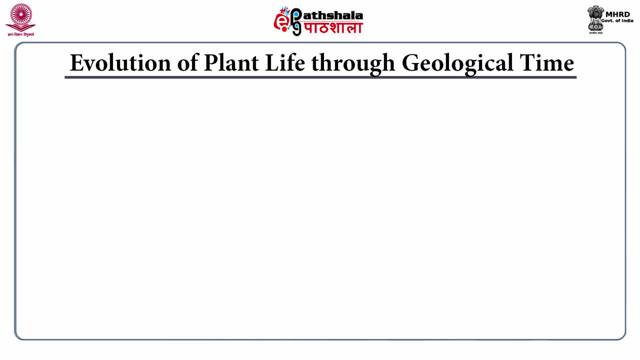 Then evolution of plant life through geological time. Early plants were small, unicellular or filamentous, composed mostly of soft body tissue with simple or no branching factor. The oldest record of life on earth are as old as 3.2 billion years. They comprise of: 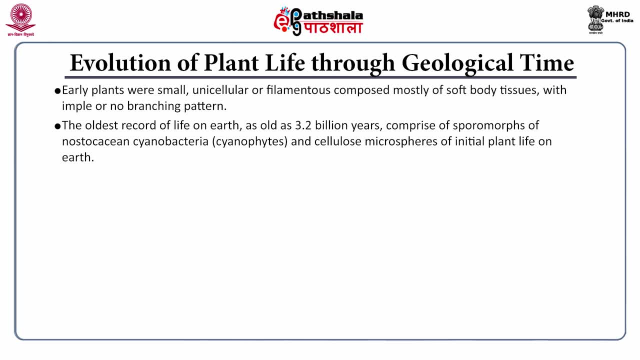 spore morphs of nostracean cyanobacteria. Students, this cyanobacteria are very interesting living form on this earth, So you try to know what are cyanobacteria. Basically, these are not bacteria, these are algae, So you try to know what are cyanobacteria and cellulose microspheres of initial plant. 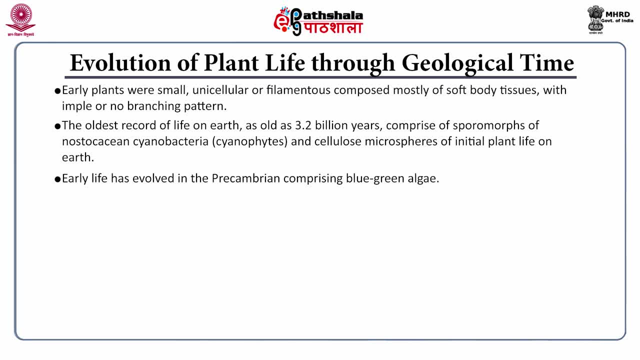 life on earth. Early life has evolved in the pre-Cambrian comprising blue green algae, and this blue green algae is nothing but cyanobacteria. There were no land plants with vascular tissue until the mid-Celerian time of the early Celerian period. 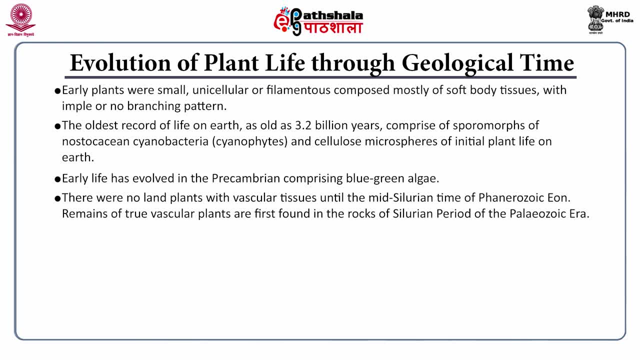 The remains of true vascular plants are first found in the rocks of Celerian period of the Paleozoic era. Early Devonian plants didn't have roots or leaves like the plants most common today, and many had no vascular tissue at all. They probably spread largely by vegetation. 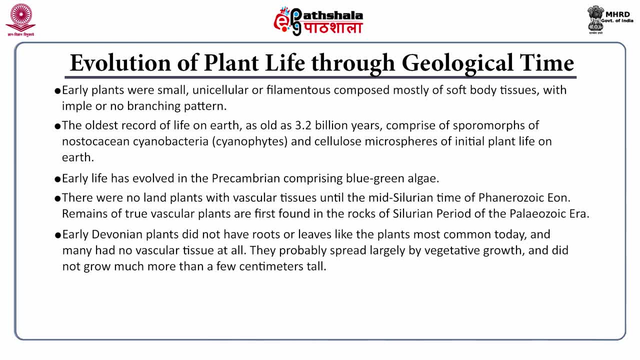 growth. They didn't grow much more than a few centimetre tall. Rheinchart, an early land plant fossil locality of Scotland, is an early Devonian deposit composed primarily of silica, having preservation of mosses and lycopodes, along with many other. 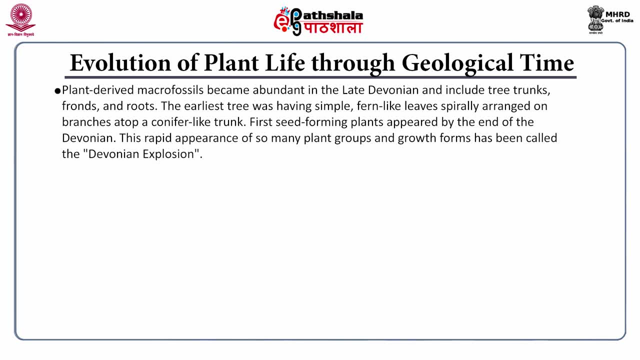 fossils. Plant-derived macro fossils become abundant in the early Celerian period. In the early Celerian period, there were only a few micro fossils. In the early Celerian period, there were only a few micro fossils. In the early Celerian period, there were only a few micro fossils. 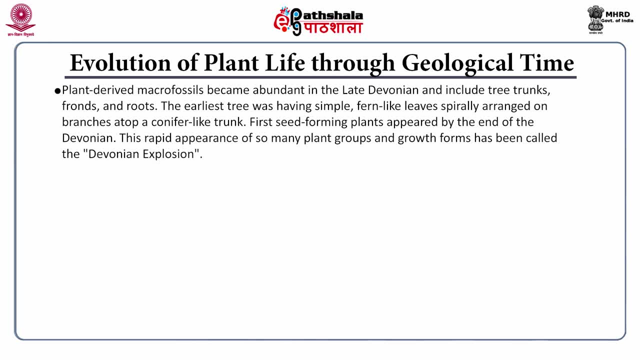 They remained abundantly in the late Devonian era and included tree trunks, fronds and roots. The earliest tree was having simple fern-like leaves spirally arranged on branches atop a conifer-like trunk. First seed-forming plants appeared by the end of the Devonian era. 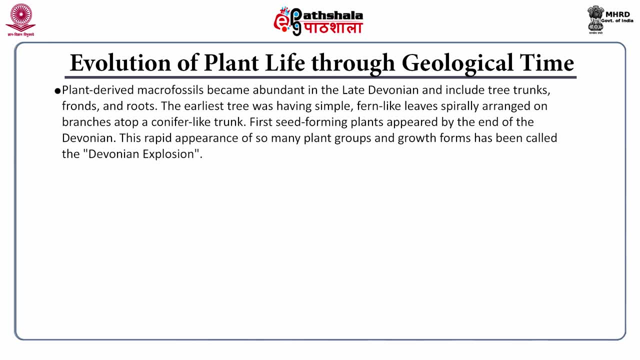 This rapid appearance of so many plant groups and growth forms has been called the Devonian explosion. The main early carboniferous plants were the horsetails. The horsetails included the common giant from calamites with a trunk diameter of 30 to 60. 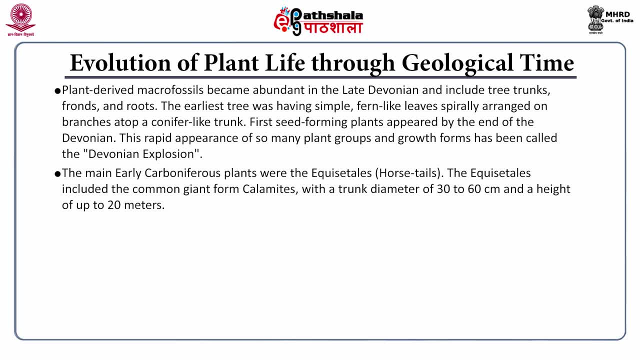 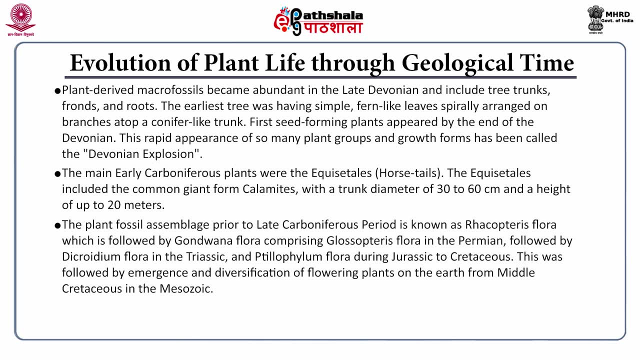 centimeter and a height up to 20 meters. The plants: the plant fossils assemblies prior to late carboniferous period is known as Rhecopteris flora, which is followed by Gondwana flora comprising Glossopteris flora in the Permian. 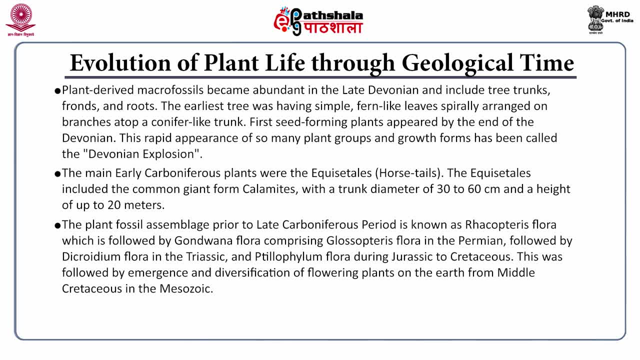 followed by Dicrodeum flora in the Triassic and Telophyllum flora during Jurassic to Persepolis. This was followed by emergence and diversification of flowering plants on the earth from middle Cretaceous in the Mesozoic, Cenozoic era has recorded the explosion of flowering plants and in the later part of 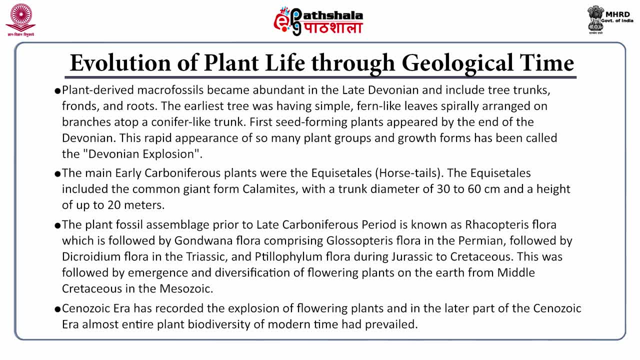 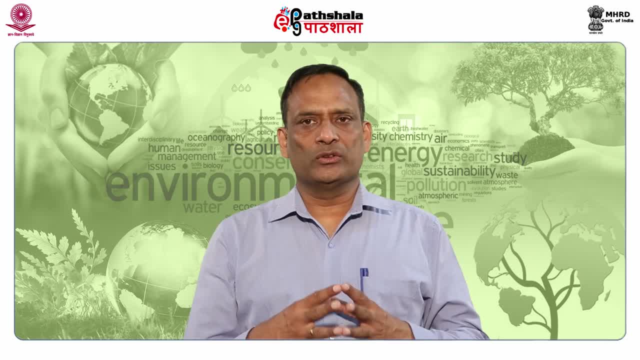 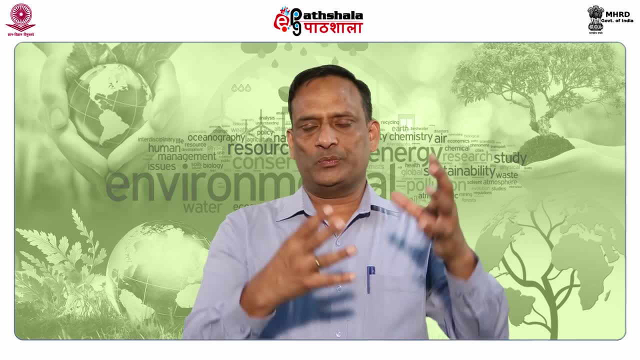 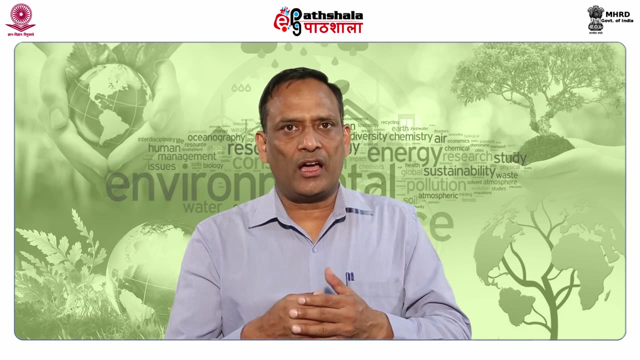 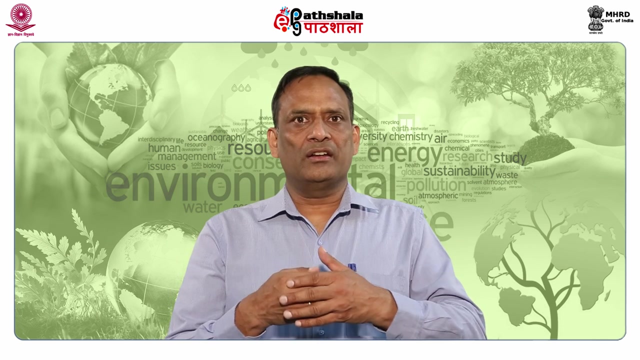 the Cenozoic era, almost entire plant biodiversity of modern time has prevailed, So this all was about paleo Botany. So in the paleo botany we have learnt that what is paleo botany and how these plant fossils can help us to know about different geological phenomena as well as we have learnt that this. 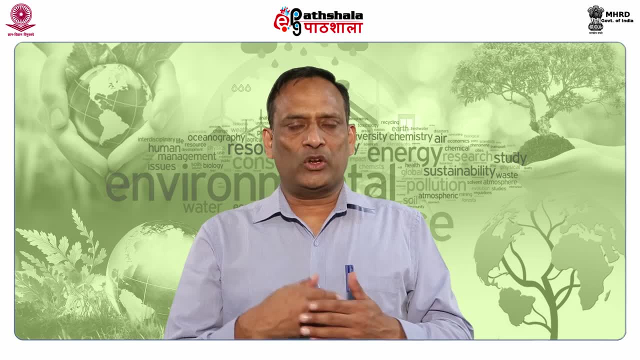 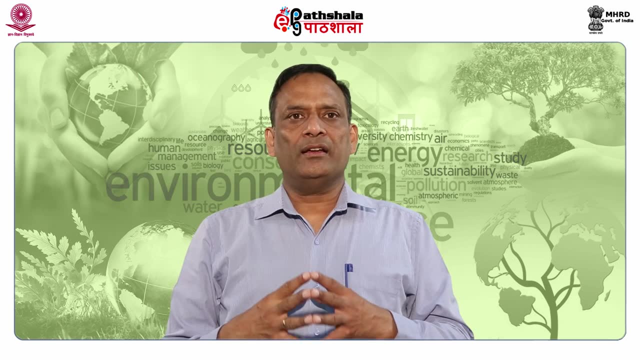 paleo botany is very, very important in petroleum exploration as well as to trace back the history of the evolution of the geological phenomena. So from our study, the second and most significant study among which we had been in the past we have resulted in is regarding the evolution of plants.